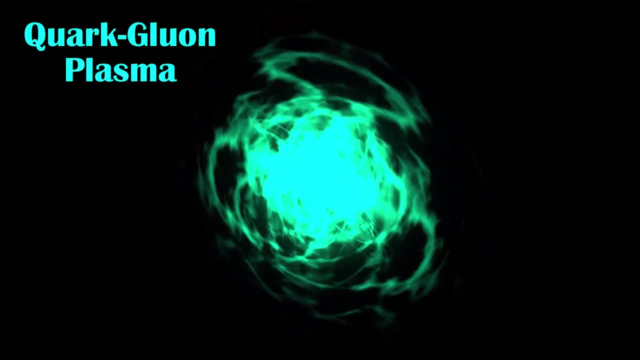 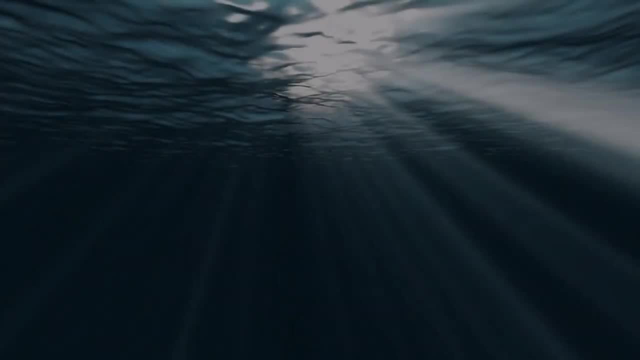 behaved relativistically, as their internal energy from the colossal temperature prevented atomic bonds from forming or the rest mass energy of particles to be comparable to their thermal kinetic energy. By relativistic I mean move with speeds almost at that of light. All particles behaved like they. 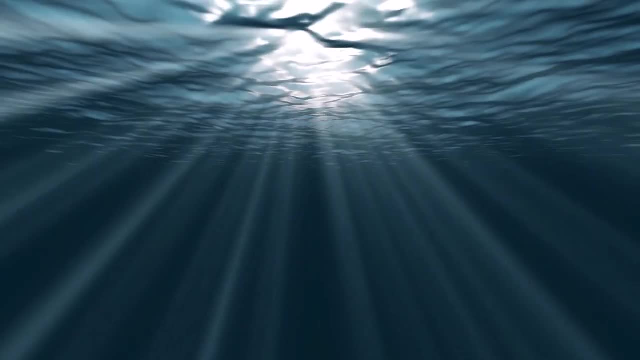 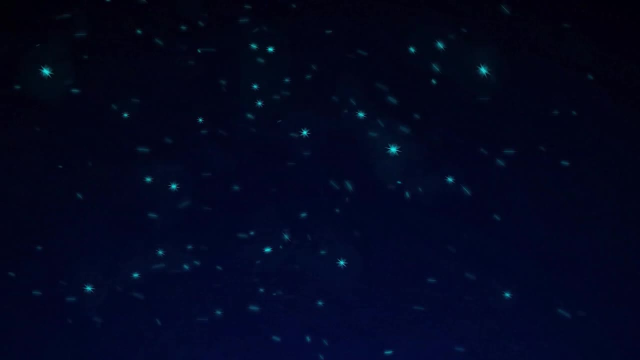 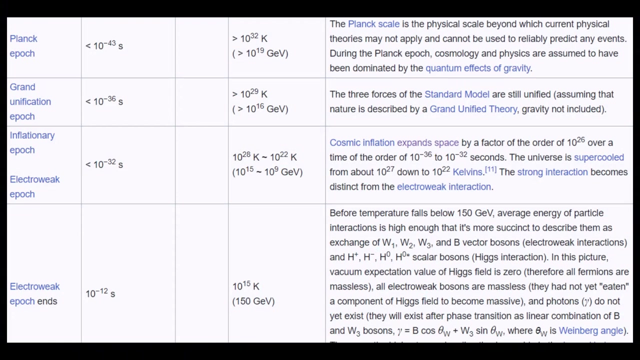 were made of photons instead of as heavy pieces of matter as we know them as today. However, as the universe continued to expand, it gradually cooled. Over time, different particle species stopped behaving relativistically, which brings us onto the different epochs in cosmic history. As different particle species cooled and stopped behaving relativistically, they stopped dominating. 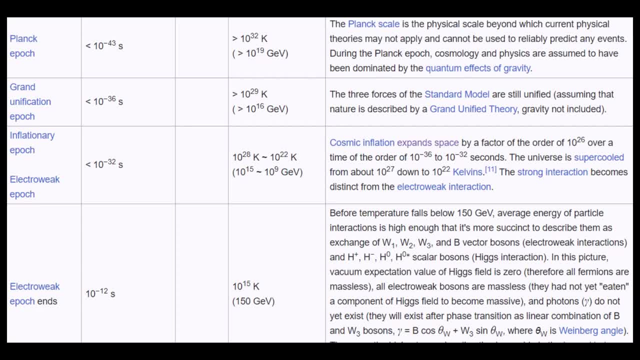 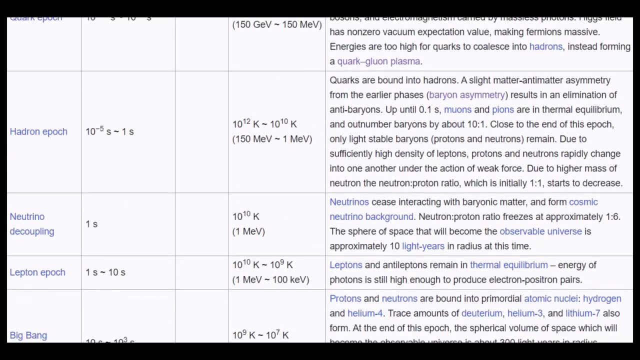 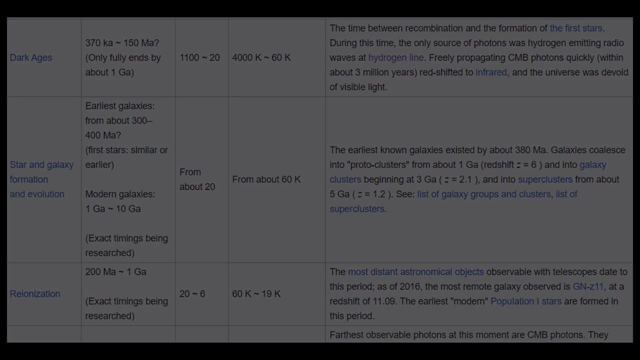 the radiation content of the universe, The average energy density of the universe decreases, which stops highly energetic particle- antiparticle species being produced. This means that eventually, the universe stopped producing certain types of particles, such as electrons, due to it cooling to a low enough temperature that it has insufficient energy to produce them. This happened in steps based 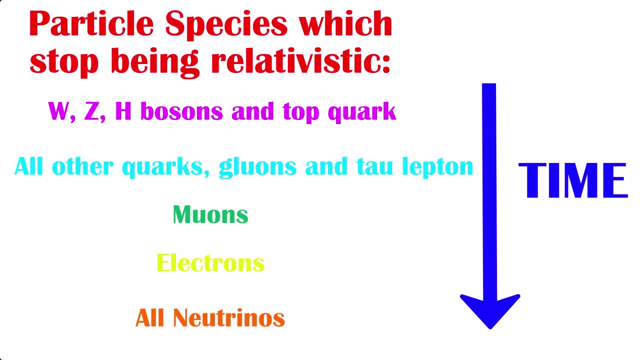 on particle mass or energy requirements. as shown on screen here, Throughout all these epochs the universe is opaque, as all of the relativistic particle species form a plasma which prevents free passage of photons. Eventually, the universe cooled enough and allowed atoms to form. By this I mean 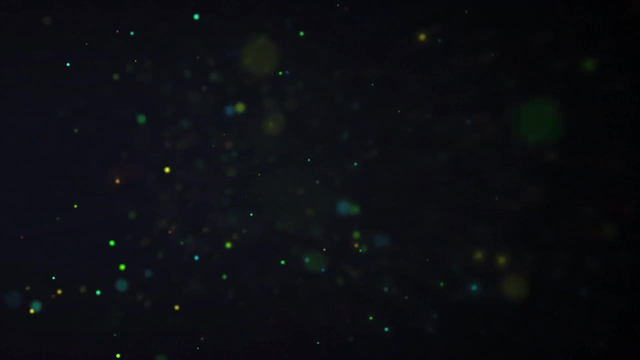 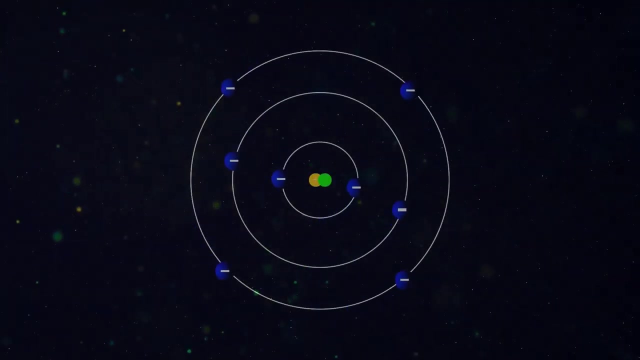 photons coupled with protons From this moment to the present day marks the photon epoch, Named this way as photons remain the only particles to be truly relativistic still in the universe. At the start of this epoch, the universe stopped being opaque. This is known as recombination. 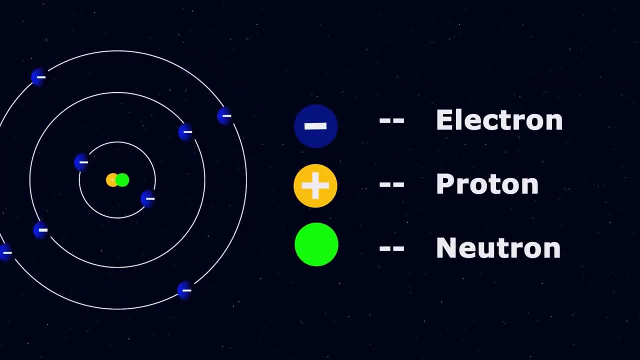 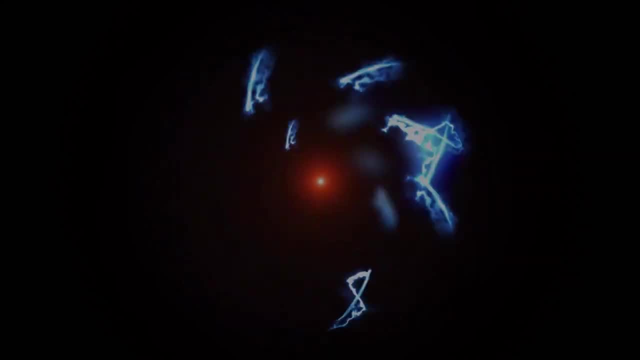 At the point of recombination, neutral atoms formed, which releases even more photons. This is known as decoupling and, as most neutral atoms are transparent to most wavelengths of light, these photons released during recombination can still be seen and detected today, and is what makes up the evolution of the universe. This is what makes up the evolution of the universe. 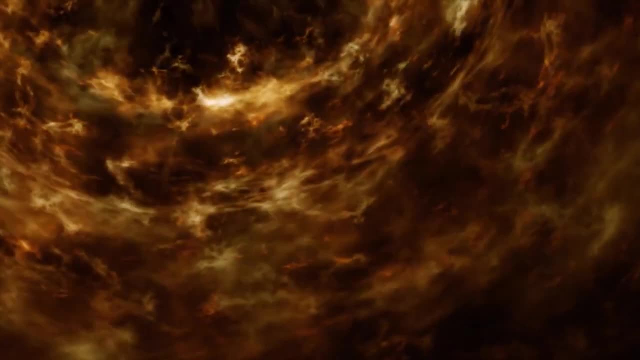 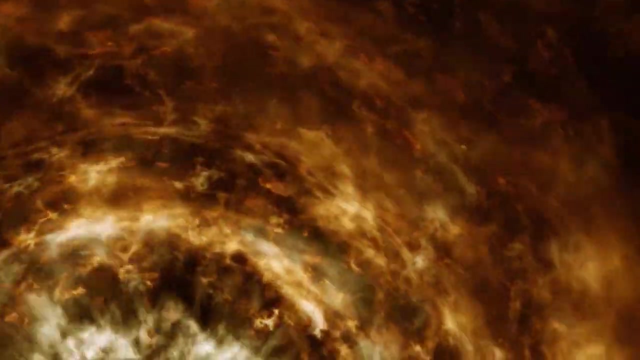 the cosmic microwave background. So the CMB is an opaque boundary which covers up and stops us from observing the earliest times in the universe, when it was so hot that electrons and protons weren't coupled. Obviously, this isn't the easiest idea to visualize, so let me give you an analogy. 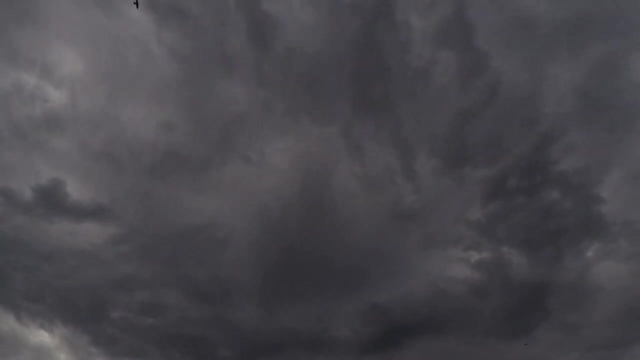 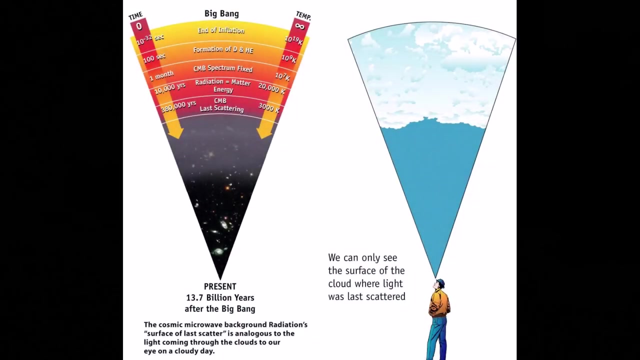 Think about the sky on an overcast or very cloudy day. You can't see what's higher up or beyond the clouds, since the clouds are obviously opaque. The clouds in this visualization are analogous to the CMB radiation: It's an opaque layer which doesn't lessen. 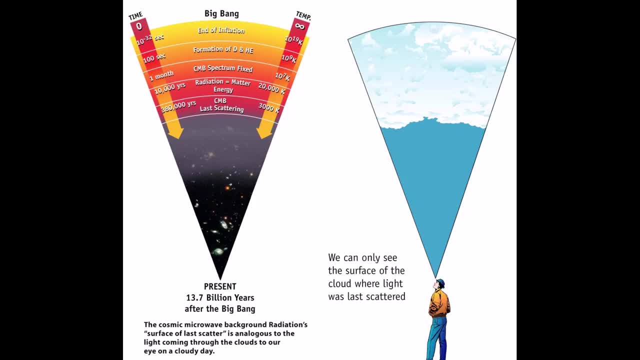 the distance between the clouds and the CMB. The CMB is mostly isotropic and homogeneous, unlike clouds, and the biggest difference between this analogy and the CMB is that, rather than the CMB blocking things that are beyond a certain distance away, it's concealing things that are 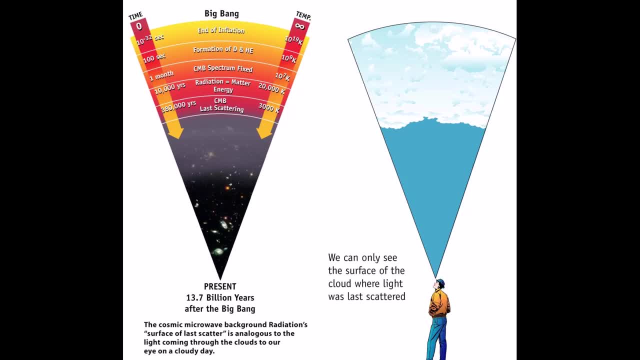 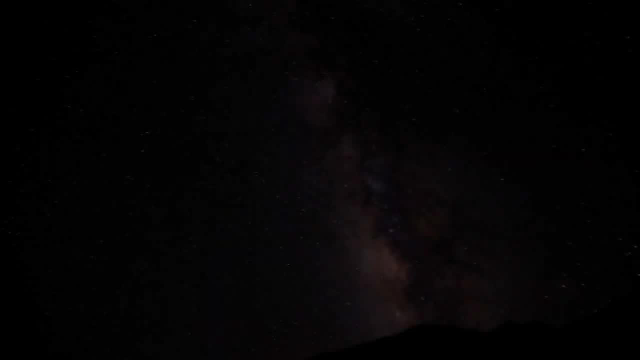 a certain time period away, As in cosmology, when you're observing light from far distances across the universe, you're really seeing what it looked like at the time said light was emitted. So the CMB is preventing us from seeing back further in time than when neutral atoms formed, As I meant. 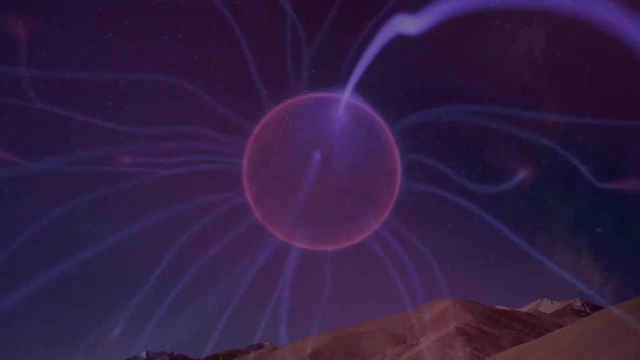 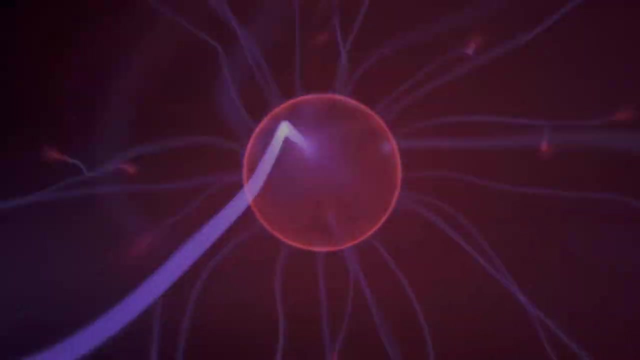 this process released photons which formed the CMB spectrum. Back then the photons released had high energy, but due to cosmological redshifting, the energy of CMB photons has decreased to a point where it's now in the microwave part of the electromagnetic spectrum. Microwaves are low energy. 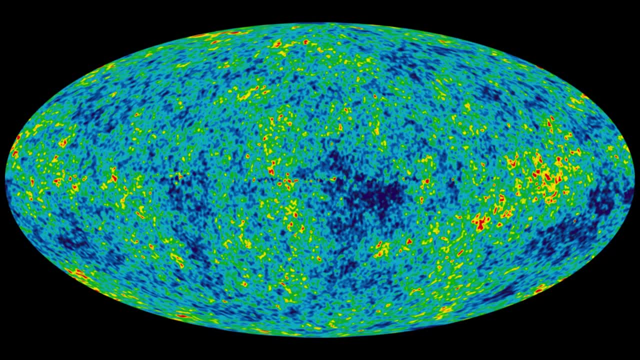 light waves and are the same as what's used to heat up your food. So this image is really a picture of what the early universe looked like at the time of recombination, after taking into account the redshift. Well, not exactly. Thing is images like these are taken. 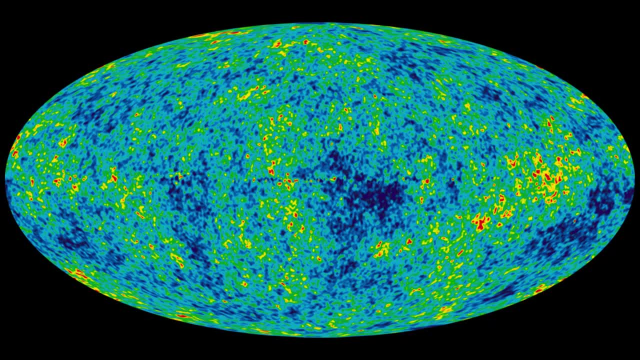 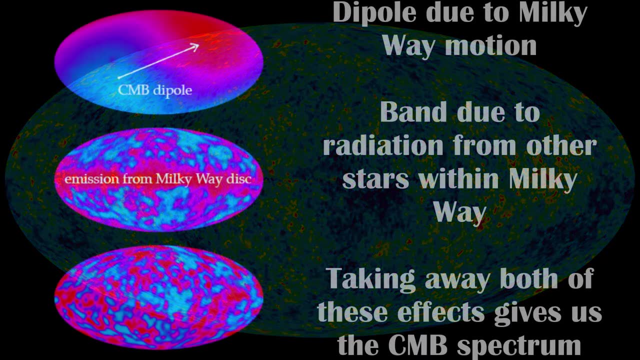 from detectors such as Planck and have been heavily processed. First off, when surveying the night sky, there's lots of other things in the way of our detectors and the pure CMB photons, Things such as the dipole caused by the movement of the Milky Way galaxy, as well as all the radiation. 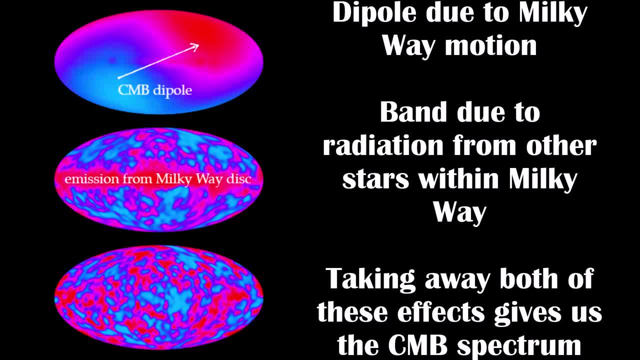 emitted from the Milky Way itself. These things interfere with our images of the CMB, and so scientists use computers to model them and then remove them from the final image. Showing on screen now is what the CMB spectrum really looks like before processing. You can see the dipole. 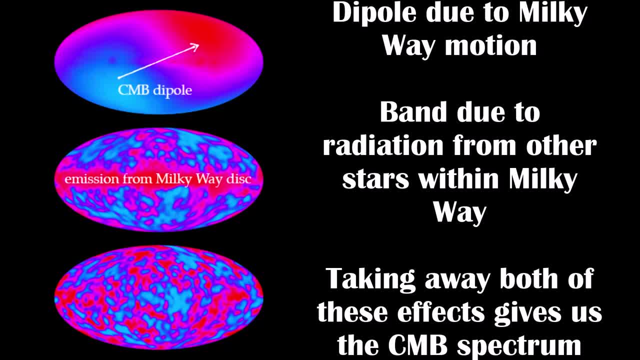 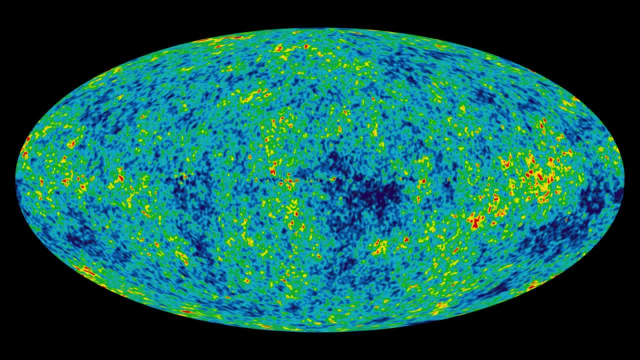 is the effect of the relative motion through the Milky Way and also the horizontal band of radiation where the Milky Way has contaminated the readings. When you take effects like these away, you get back to the well-known CMB image. However, that's not the only thing done to it. 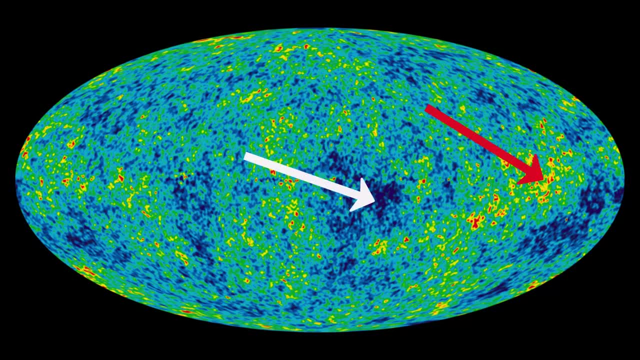 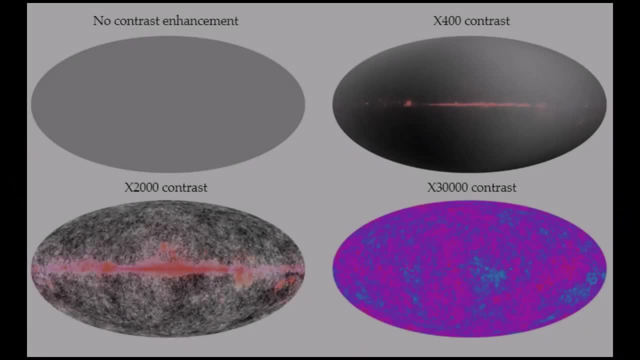 Although it may seem that there's places of really cold and really hot regions shown in red and blue, that isn't actually the case. While the colour coordination does indeed show relatively where's hotter and where's colder, the temperature differences between the reddest part and the 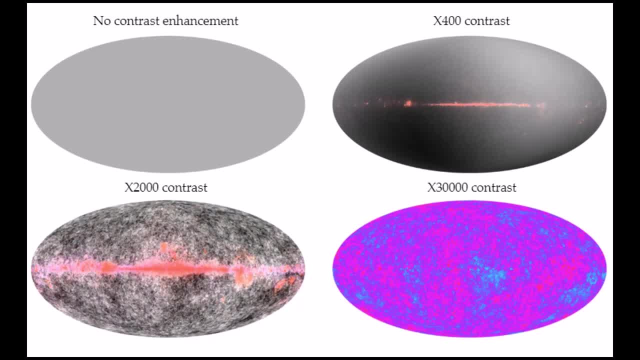 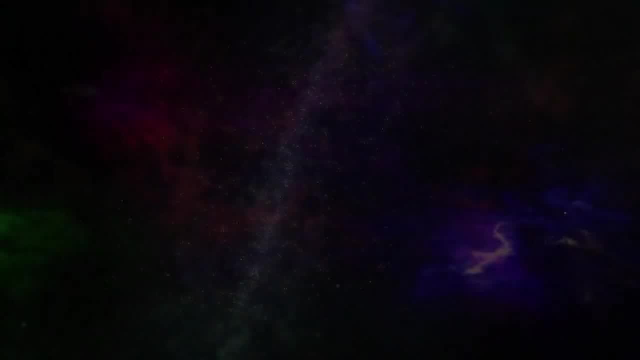 bluest part is only around one in a thousand of the three, With the average CMB temperature being about 2.7 kelvin or minus 270.4 degrees celsius. Key assumptions of the universe is that it's homogeneous and isotropic, meaning that every 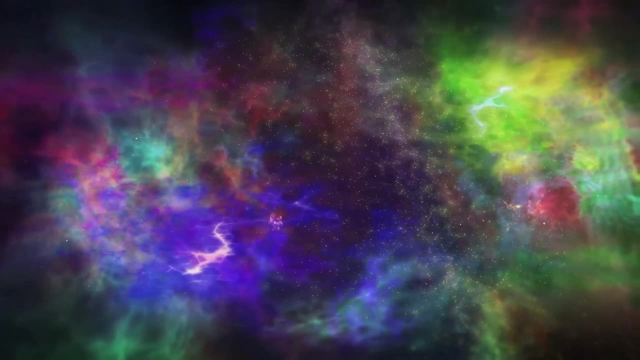 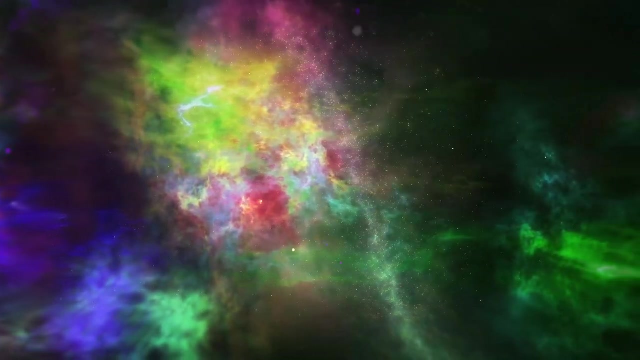 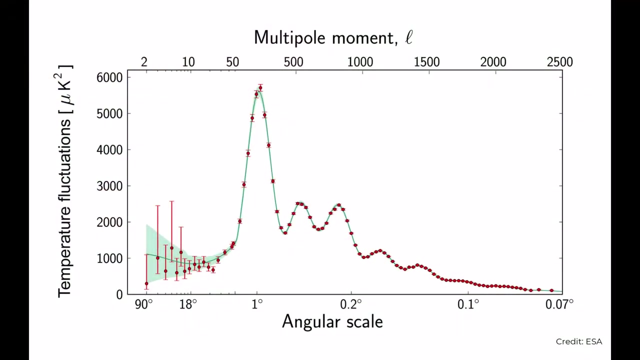 point is the same and everywhere you look you should see the same thing. The CMB is key supporting evidence for those two assumptions. but the temperature differences or anisotropies in the spectrum show that the universe isn't perfectly isotropic. I must stress that this isn't a bad thing, quite the opposite. The distribution of temperature. 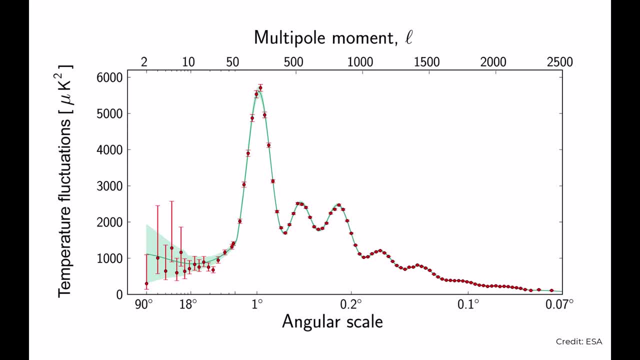 and isotropy can be used by cosmologists to test models for the universe. This is essentially what the Planck satellite mission was for. All of the CMB spectrum data can be compared to computer models of the universe and what they predict the CMB spectrum to look like. If the initial 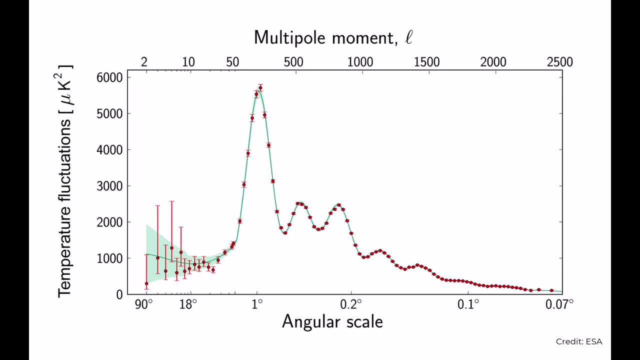 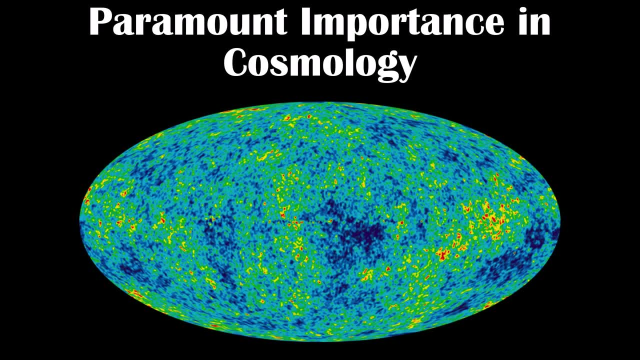 conditions or parameters. create a model CMB spectrum which closely matches the one we see in our universe, then we know that those initial conditions must be close to reality. So the CMB acts as a really powerful tool which allows us to probe the early universe and its 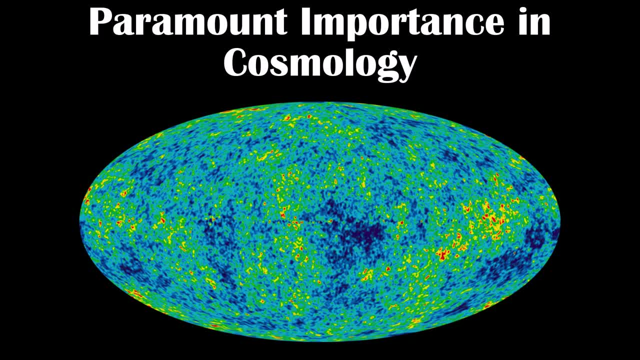 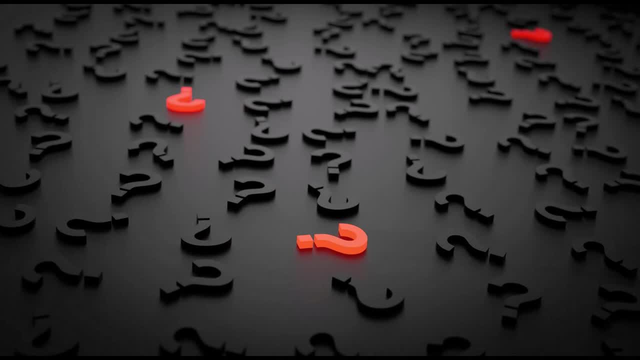 conditions. It acts as evidence in support of a hot big bang, a flat universe and probably also a cosmological constant form of dark energy. If those terms are unfamiliar to you, you may wish to check out my other videos where I discuss other parts of cosmology in more depth. So let's review. 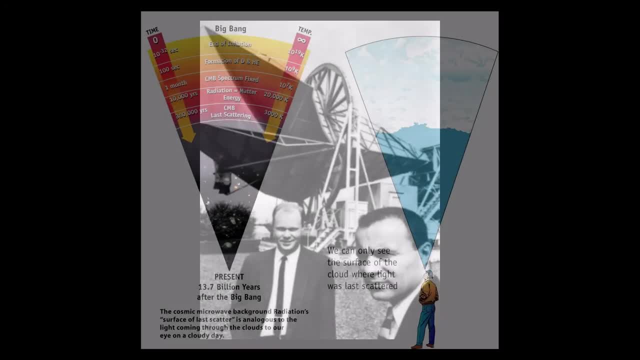 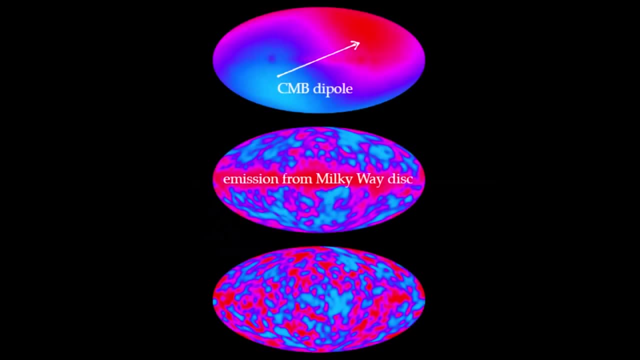 The CMB was accidentally discovered in 1964 and is the final scattering surface of the early universe, when it was opaque and neutral atoms had just formed. The image shows the universe's anisotropy after effects from the Milky Way radiation band, and dipoles have been removed. 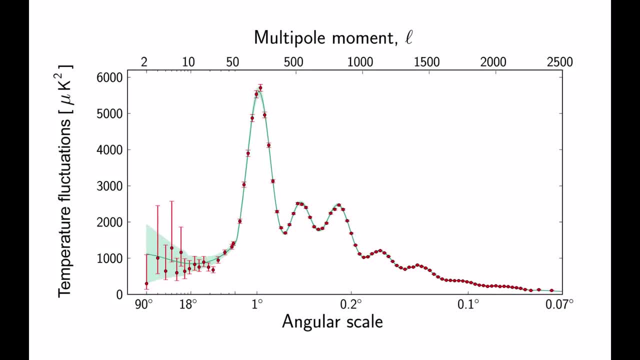 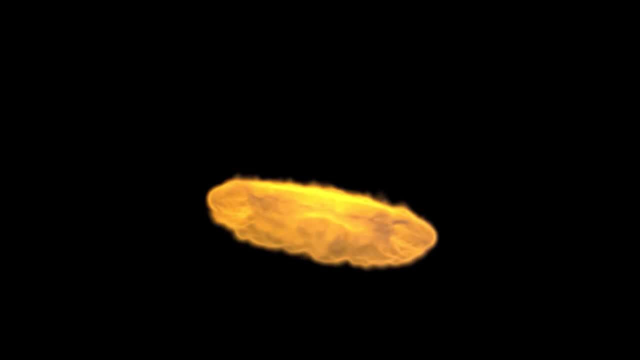 It shows the universe to be mostly homogenous, but the distinct differences allow cosmologists to probe the early universe and accurately test mathematically its initial conditions. If you've enjoyed this video or learned something new, please consider liking and subscribing. Only a small percentage of people who watch my videos are actually subscribed. 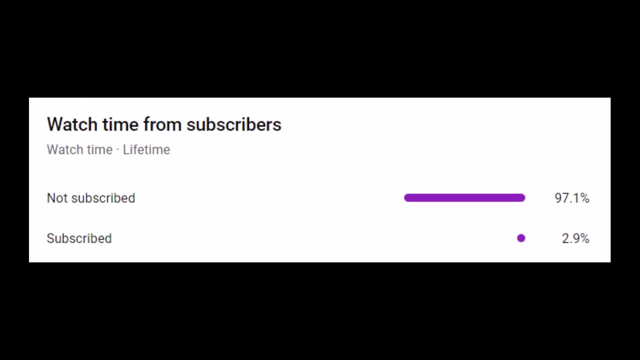 It's free. it helps out my channel a bunch and you can always unsubscribe. See you next time.